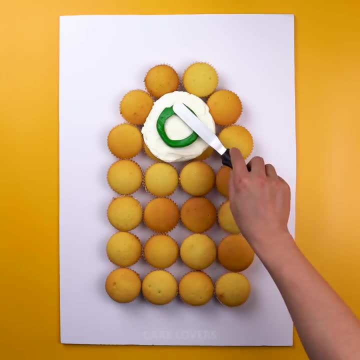 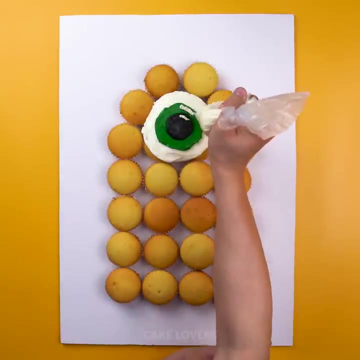 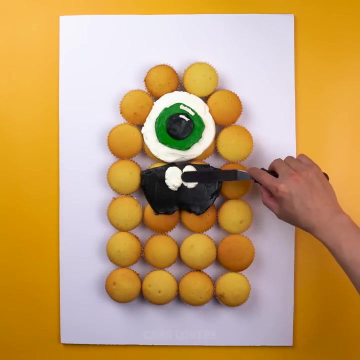 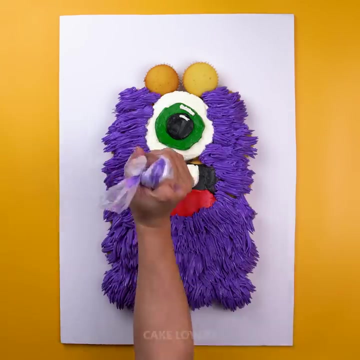 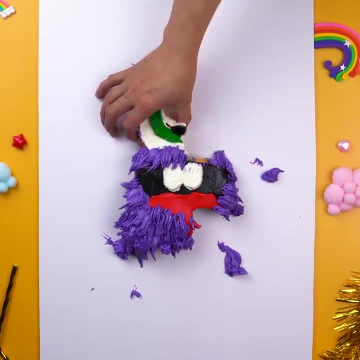 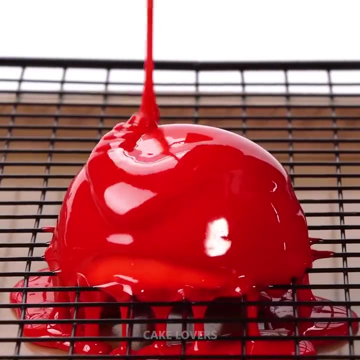 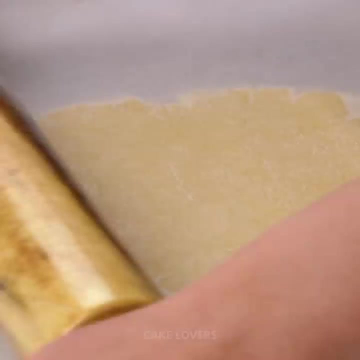 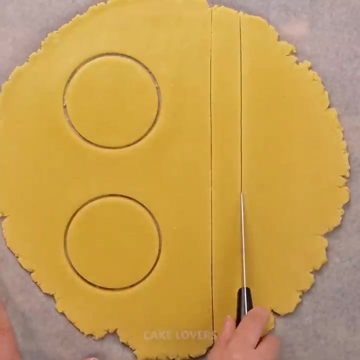 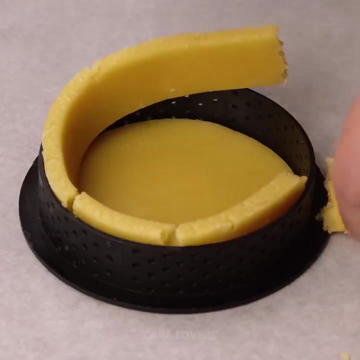 We fall apart piece by piece. That's how the little things get huge. Just keep on moving through the beat. Don't let them get the best of you When you are under the weather, Getting caught in the storm. Do you remember I told you, if we dance in the blizzard, 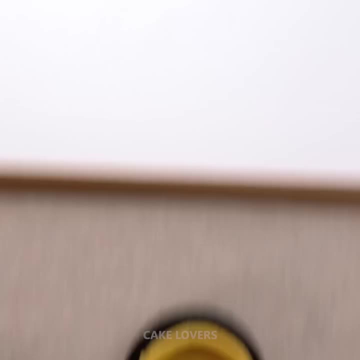 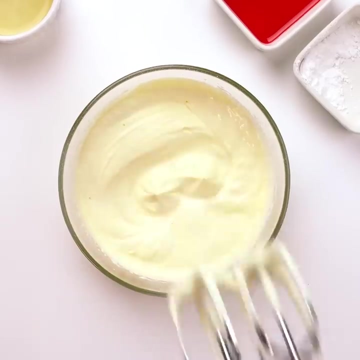 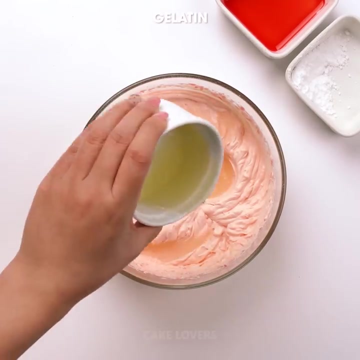 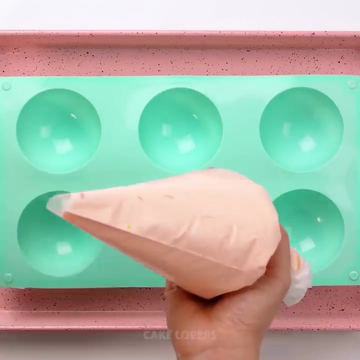 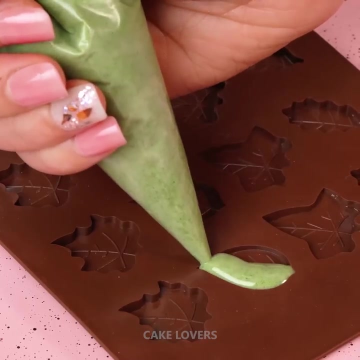 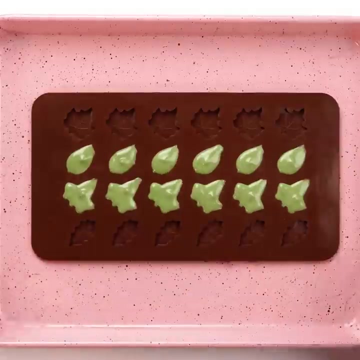 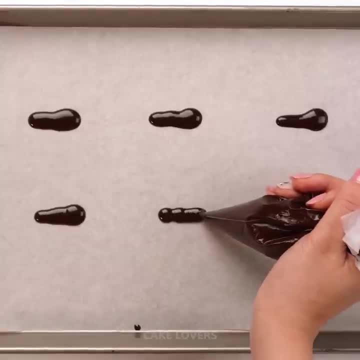 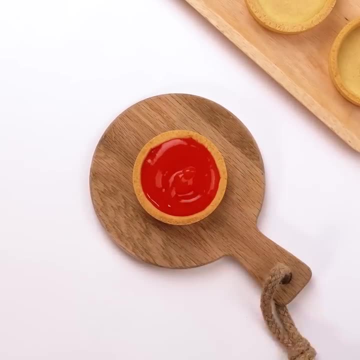 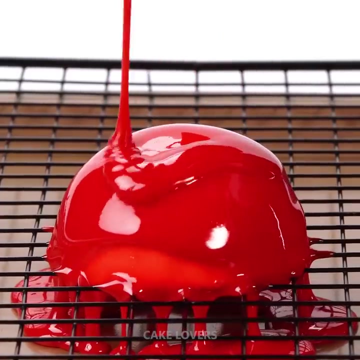 Your name lighting up the screen, But you never call. when you're sober You say you don't like the games, But you play me like there's no tomorrow. You should know that I'm fed up with your lies, so don't come closer. You know you hurt me bad and I have scars. 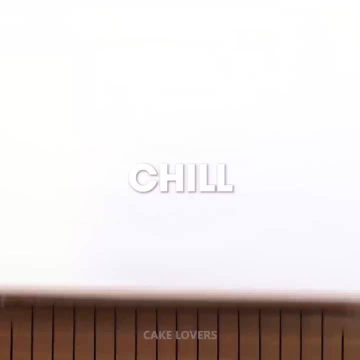 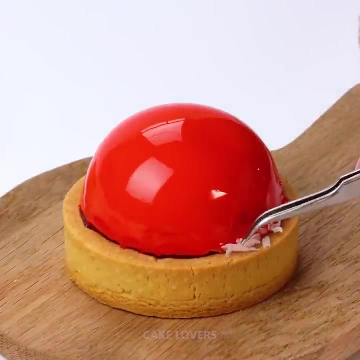 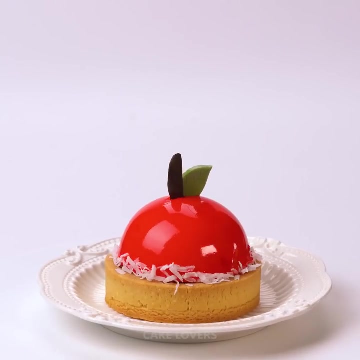 I need some time to heal, so don't come over, Don't even bother calling, just get lost. I'm fine on my own. So don't even bother to come back, Cause I ain't done. I'm fine on my own, And boy, you're a pretty little lie. 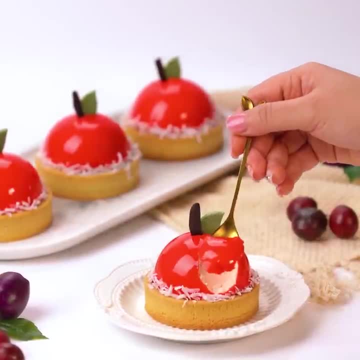 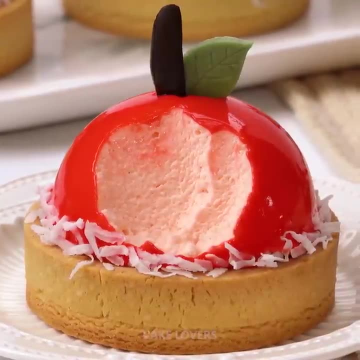 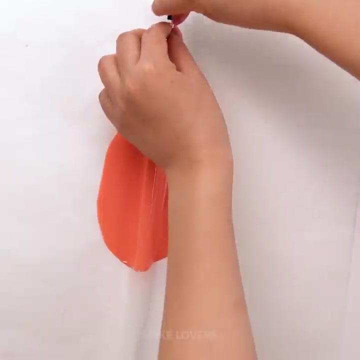 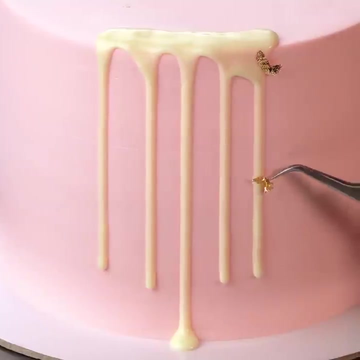 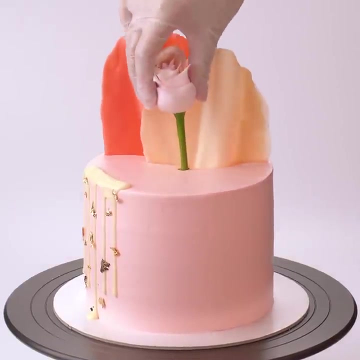 As it's getting old. All the nights I have wasted on you Are gone cause we are through. All the nights I have wasted on you Are gone cause we are through. You say you don't wanna be your thing, But I'm not the one who's calling. I'm tired of waiting For you to change into someone, Someone who could love me, But you play me like there's no tomorrow. You should know that I'm fed up with your lies, so don't come closer. You know you hurt me bad and I have scars. 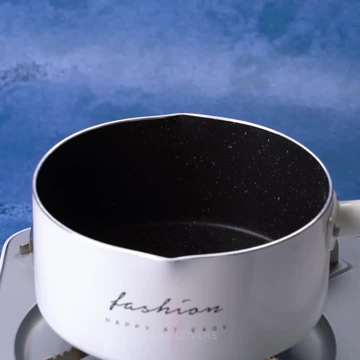 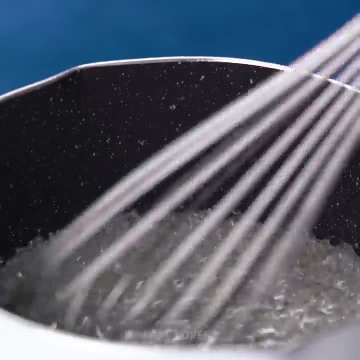 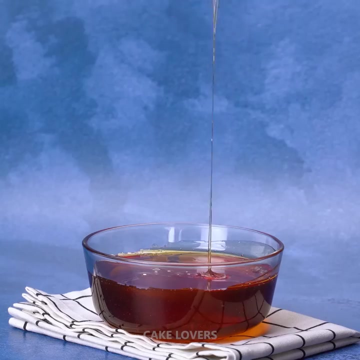 I need some time to heal, so don't come over, Don't even bother calling, just get lost. I'm fine on my own. So don't even bother to come back, Cause I ain't done. I'm fine on my own, And boy, you're a pretty little lie. 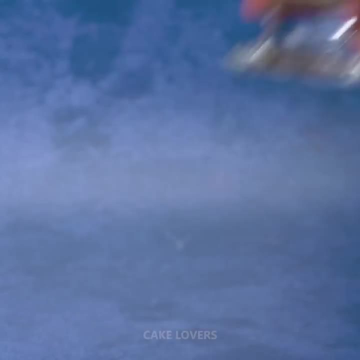 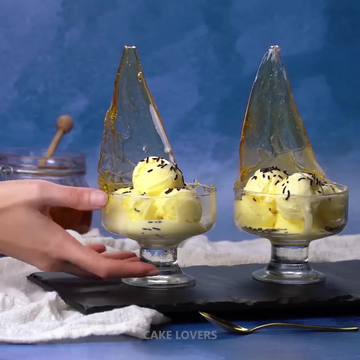 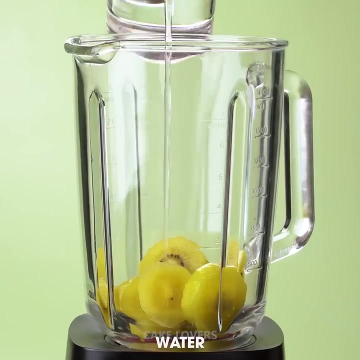 As it's getting old, All those late nights I've waited for you Are gone, cause we are through. All those late nights I've waited for you And boy, you're a pretty little lie, As it's getting old. All those late nights I've waited for you. 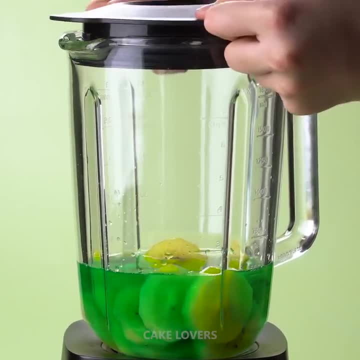 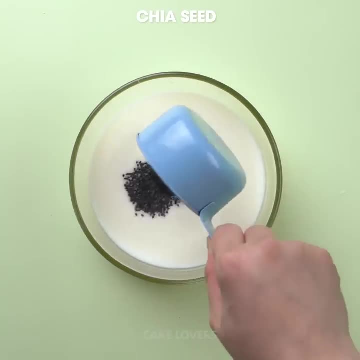 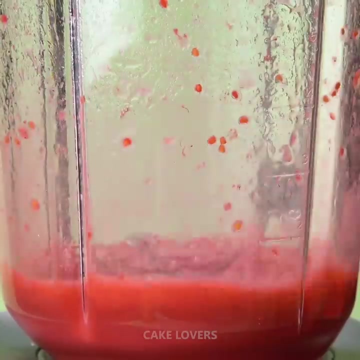 Are gone cause we are through. Your lies are getting old. I'm getting stronger. You think that my bed's getting cold, But it's feeling warm. Your lies are getting old, But I'm getting stronger. I'm getting stronger Cause I'm fine on my own. I'm fine on my own. 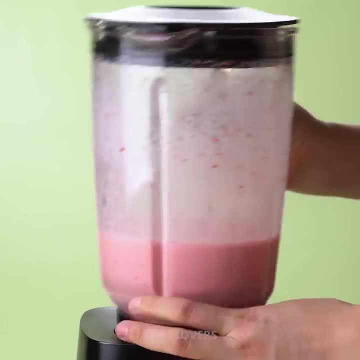 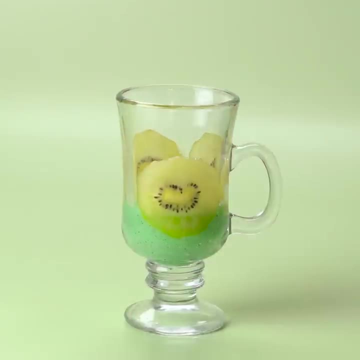 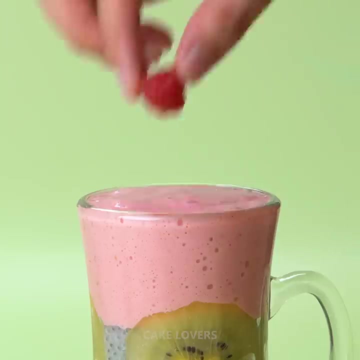 So don't even bother to come back, Cause I ain't done. I'm fine on my own. And boy, you're a pretty little lie, As it's getting old. All those late nights I've waited for you Are gone, cause we are through. All those late nights I've waited for you. 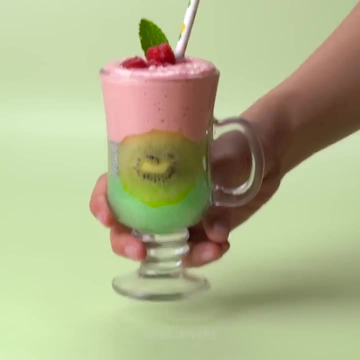 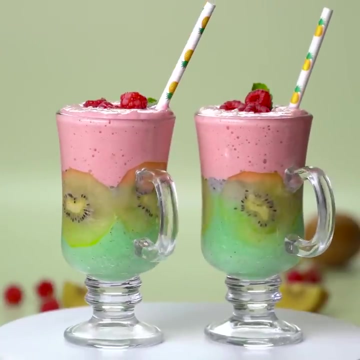 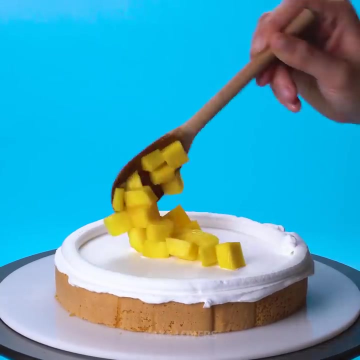 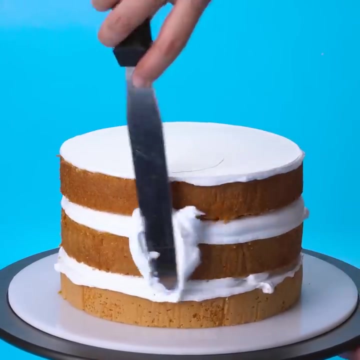 Are gone, cause we are through, Cause we're through. Gotta get, Gotta get. Gotta get it right now. Yeah, push all the limits with you right now. Gotta get it right now. Yeah, push all the limits with you right now. Yeah, push all the limits with you right now. 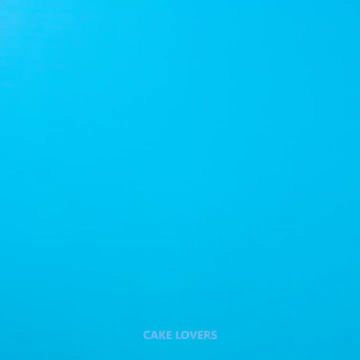 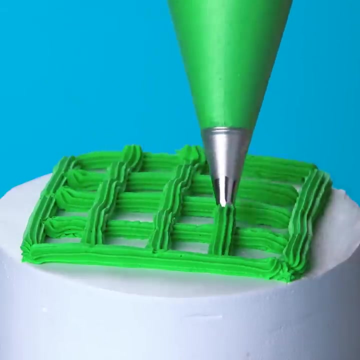 Yeah, push all the limits with you right now. Gotta get it right now. Yeah, push all the limits with you right now. Yeah, push all the limits with you right now. Yeah, push all the limits with you right now. Gotta get it right now. 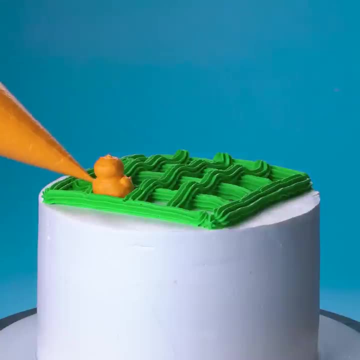 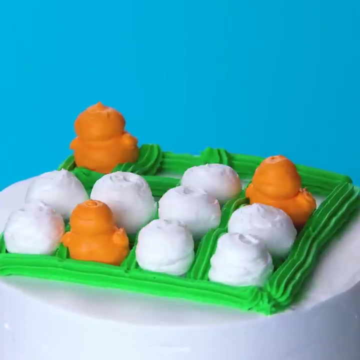 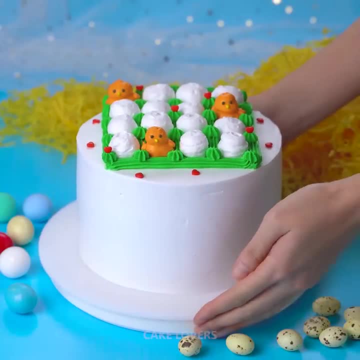 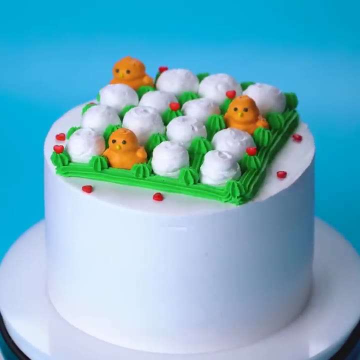 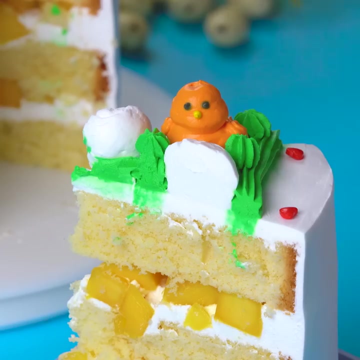 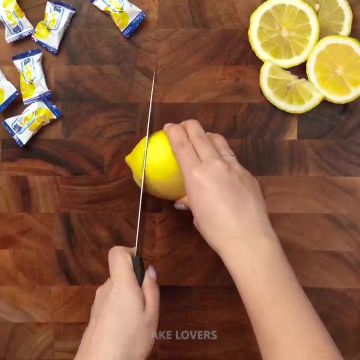 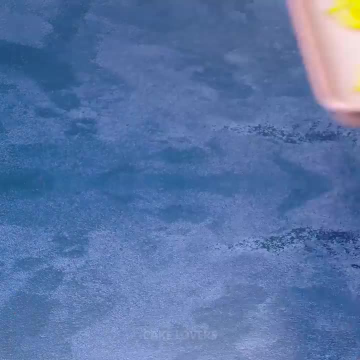 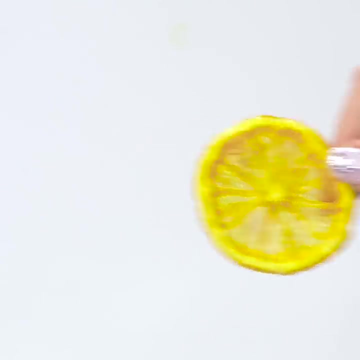 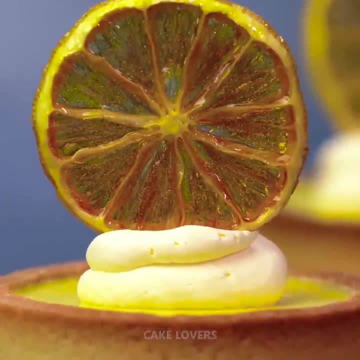 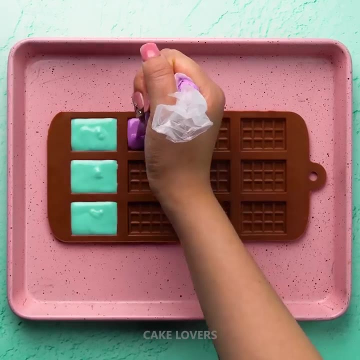 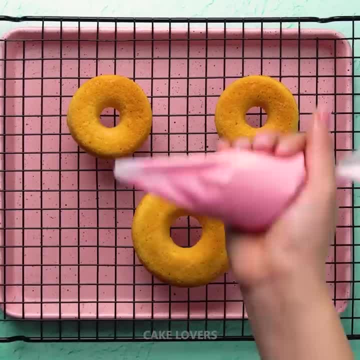 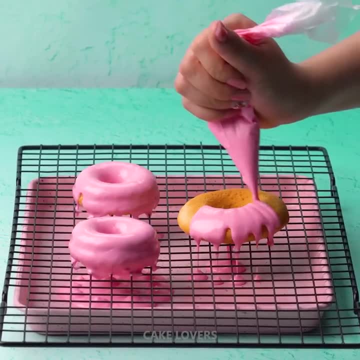 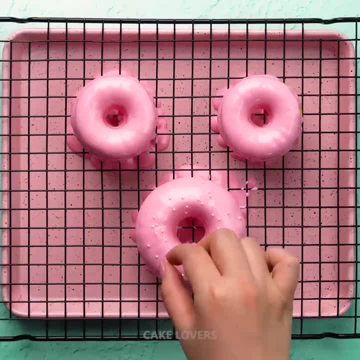 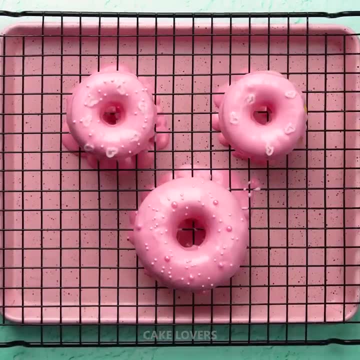 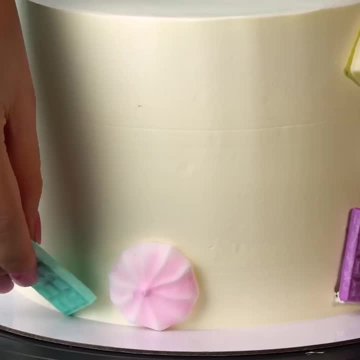 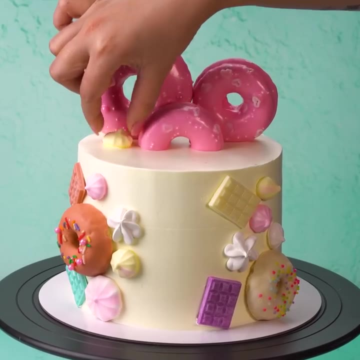 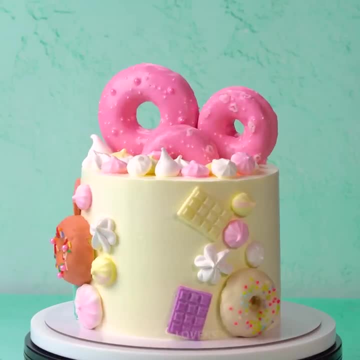 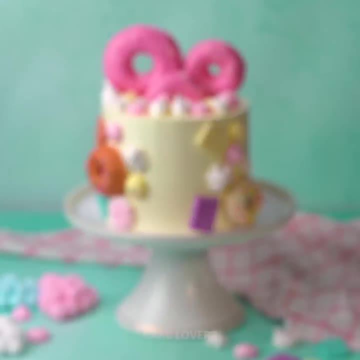